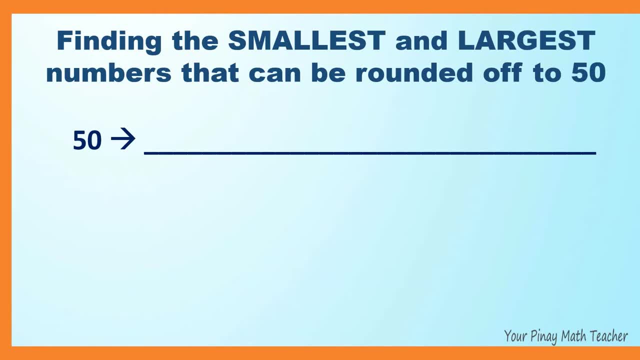 How to find the largest and smallest numbers that can be rounded off to 50?. Look at the number line Between 40 and 50 is 45. It reaches the middle. Therefore, 45 should be rounded off to 50.. Similarly, 55 should be rounded off to 60. 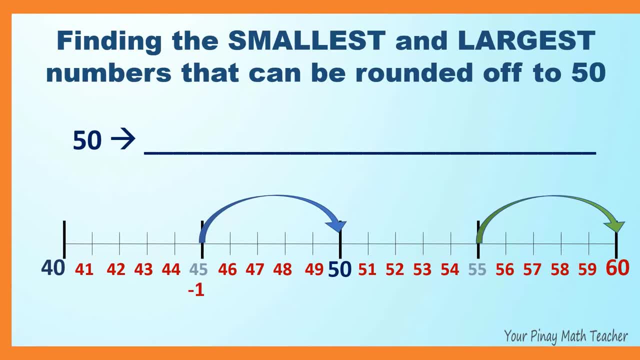 If we subtract 1 from 45,, we get 44. And since it does not reach the middle anymore, then 44 should be rounded off to 50. Same with 55. If we subtract 1 from it, it becomes 54.. 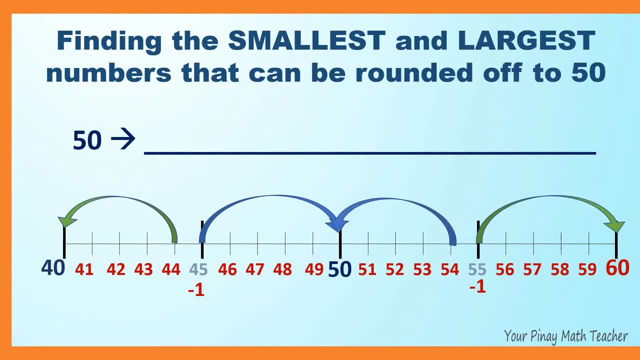 54 should be rounded off to 50.. Based on this illustration, the numbers that can be rounded off to 50 is from 44 to 50.. So the numbers that can be rounded off to 50 is from 45 to 50.. 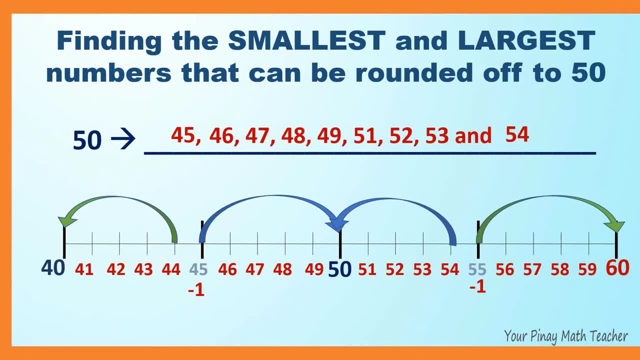 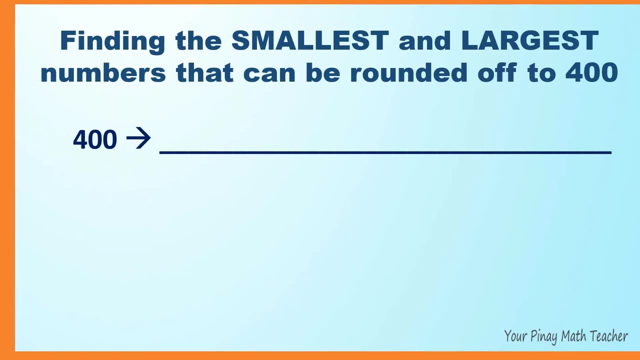 45 up to 54. Therefore, the smallest is 45 and the largest is 54. These are the numbers that can be rounded off to 50.. How about the smallest and the largest numbers that can be rounded off to 400?? Again, let's take a look at the number line Between 300 and 400 is 350. It reaches the 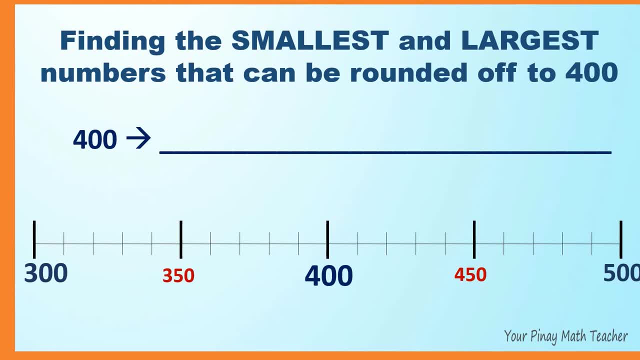 middle of 300 and 400. Therefore, it has to be rounded off to the greater 100, which is 400.. Similarly, 450 is to be rounded off to 500.. If we take 1 from 350, which is 349,. 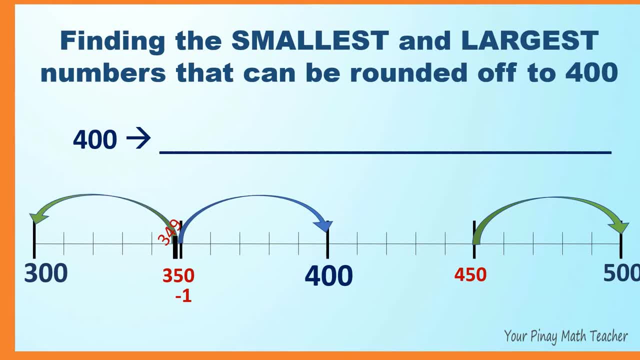 then it's to be rounded off to 300.. 450 minus 1 is 449.. It should not be rounded off to 500 because it is a number line. It has to be rounded off to 300.. So it has to be rounded off to. 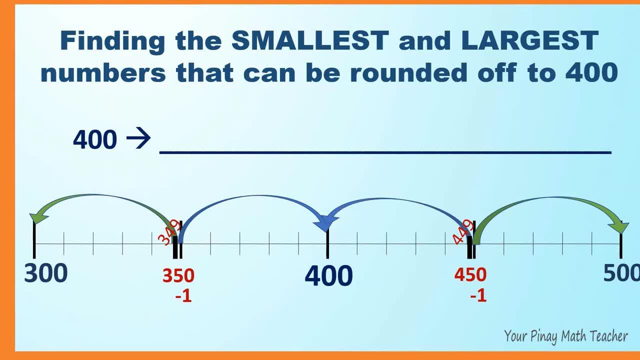 400 anymore, but to 400.. Based on the illustration, these are the numbers that can be rounded off to 400.. From 350 up to 449.. Therefore, the smallest is 350 and the largest is 449.. Next find the. 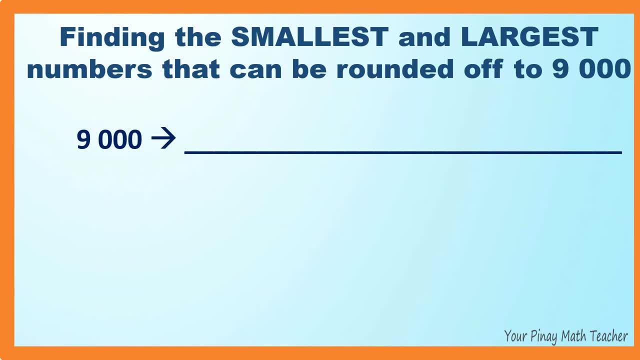 smallest and the largest numbers that can be rounded off to 9000.. Again, look at the number line In the middle of 8000 and 9000 is 8500.. Once the number reaches the middle it has to be rounded off to the greater number. So 8500 is rounded off to 9000. 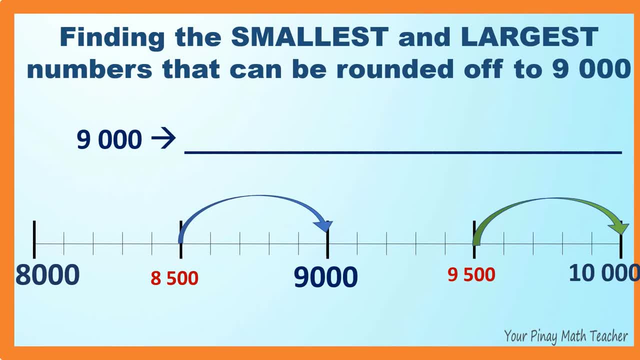 9500 is to be rounded off to 10,000.. If we take 1 from 8500, we get 8,499, which must be rounded off to 8,000.. If we take 1 from 8,500, we get 8,499, which must be rounded off to 8,000.. 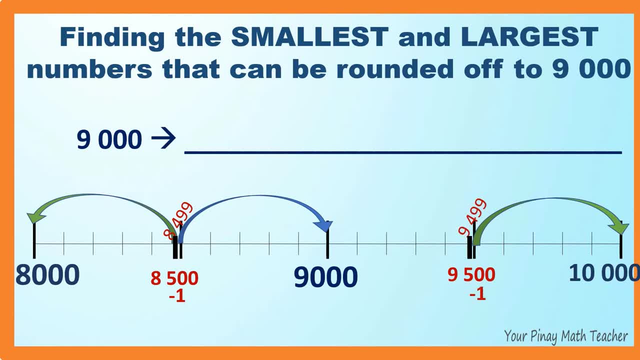 If we take 1 from 9500, we get 9,499, which must be rounded off to 9,000.. These are the numbers that can be rounded off to 9,000.. It starts with 8,500 up to 9,499.. The smallest is 8,500 and the largest 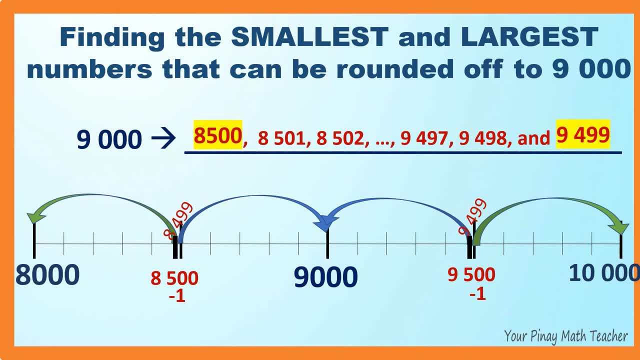 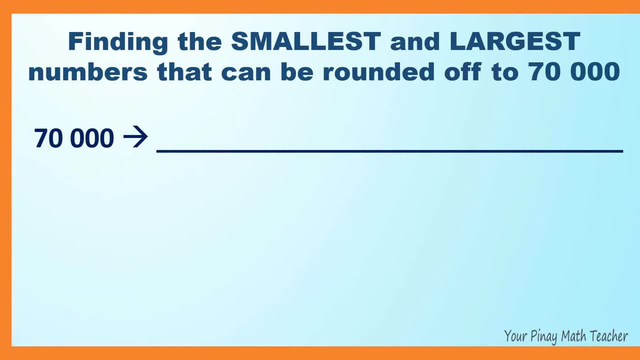 is 9,499.. four hundred ninety nine. how about the smallest and the largest numbers? that can be rounded off to seventy thousand. so, based on our number line between sixty thousand and seventy thousand is sixty five thousand, which can be rounded off to seventy thousand. seventy five thousand also, which? 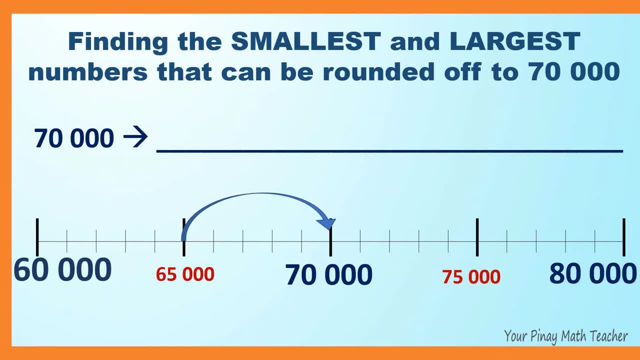 is in the middle of seventy thousand, and eighty thousand should be rounded off to eighty thousand. so if we subtract one from sixty five thousand, we get sixty four thousand nine hundred ninety nine. this must be rounded off to sixty thousand. we also got seventy four thousand nine hundred ninety nine. 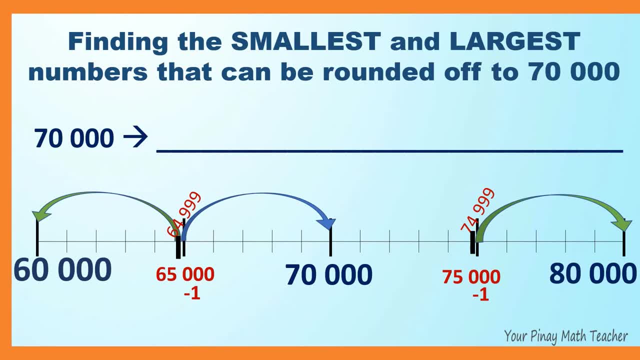 if we take one from seventy five thousand, since it does not reach the middle it has to be rounded off to seventy thousand. so the numbers that can be rounded off to seventy thousand start from sixty five thousand up to seventy four thousand nine hundred ninety nine. the smallest is sixty five thousand and the largest is seventy four thousand nine hundred.